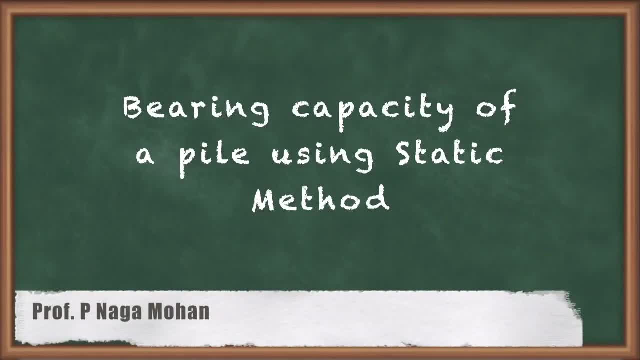 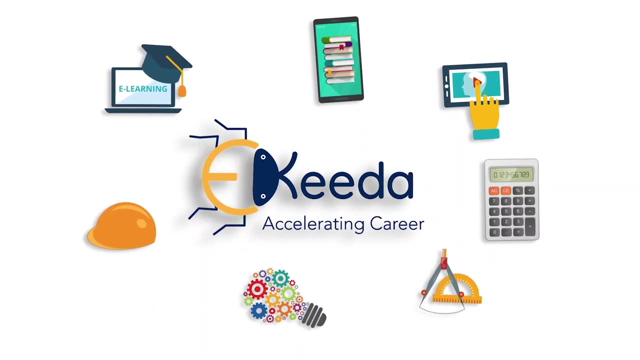 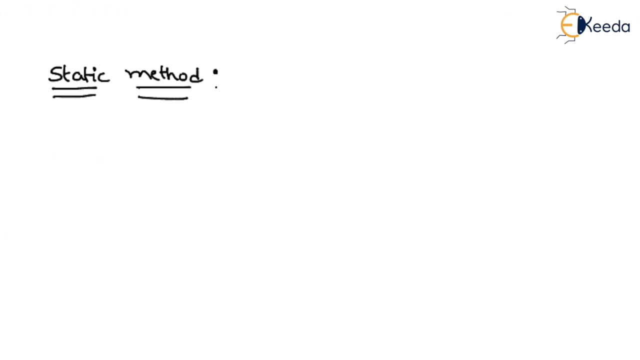 Hello friends, in the present video we will see how to find the bearing capacity of a pile by using static method. First we will discuss about the static method in general. After that we will see about the particular type of the soil. 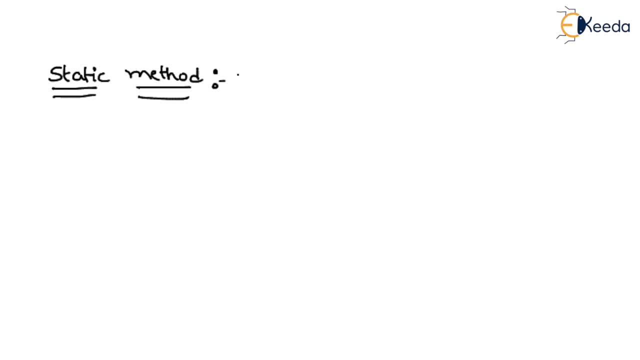 That means, if it is a sand, what is the bearing capacity? If it is a clay, how to find the bearing capacity? Okay, now let us consider a pile. It is driven through the. okay, let us assume this is the pile and up to the ground surface. 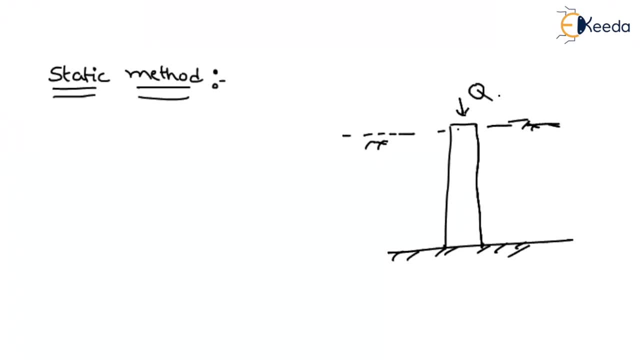 And we are applying some external load on the pile Q. Okay, in general, what is the ultimate bearing capacity of the soil, Ultimate bearing capacity of the pile, presenting by P? That will be summation of the bearing capacity because of the end bearing QB plus because of the friction, QS, isn't it? 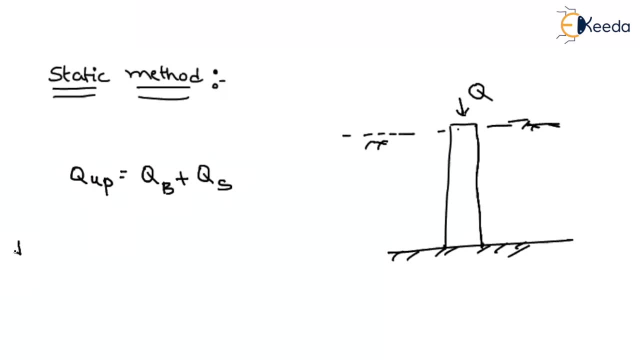 Now if it is a friction pile. if it is a friction pile, then we will consider end bearing capacity will be equal to zero If it is an end bearing pile. if it is an end bearing pile, as we have already discussed here, 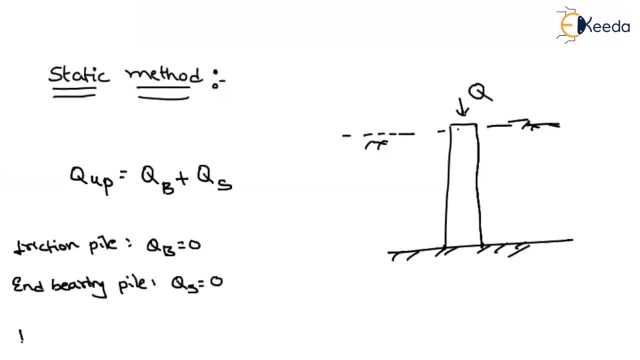 frictional capacity will be equal to zero If it is a friction cum end bearing. if it is a friction pile, what is the ultimate capacity of the pile? That will be equal to QS. If it is an end bearing capacity, what is the ultimate bearing capacity of the pile? 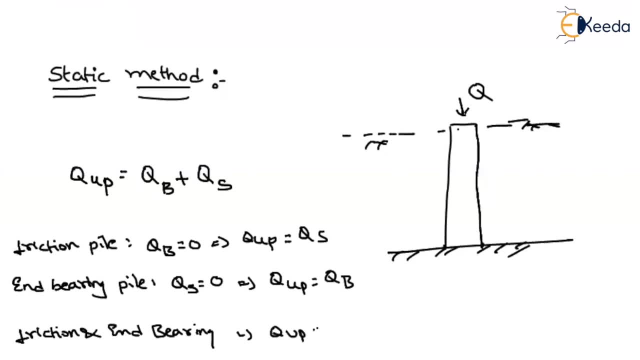 QB. If it is friction cum end bearing what is the ultimate carrying capacity of the pile, That will be equal to summation of QS plus QB. Okay now, so, depending upon the type of file, we have to consider the capacity of the file. 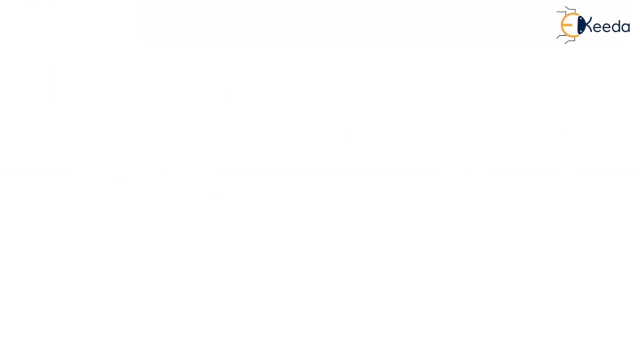 Now. so what is meant by end bearing? Isn't it Suppose I have to find capacity of the end bearing That will be QB, That will be equal to end bearing resistance, QB, into area of the end bearing. So here, QB is nothing but an end bearing resistance. 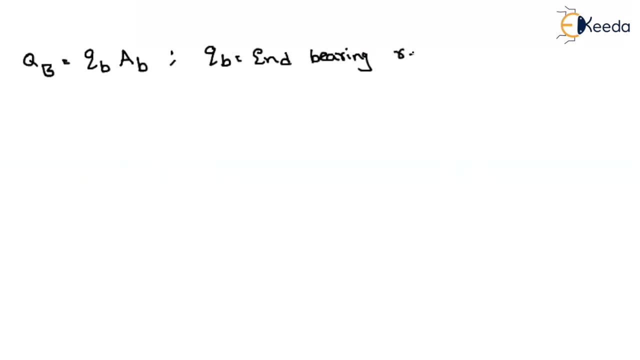 This end bearing resistance will be given in the question End bearing resistance. So if you know the end bearing resistance and if you multiply by the area at the end bearing or base area of the base of end bearing area, then we can get the end bearing capacity. 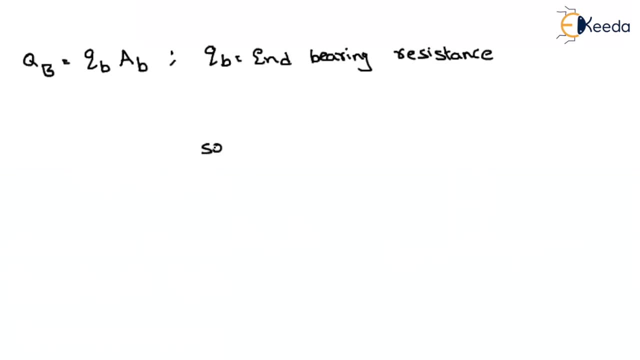 So in general, we will have the square pile and also we will have the circular pile and also we will also have the rectangle pile. Suppose, if you are talking about the square pile, What about the bottom area will look like? It will look like a circle. 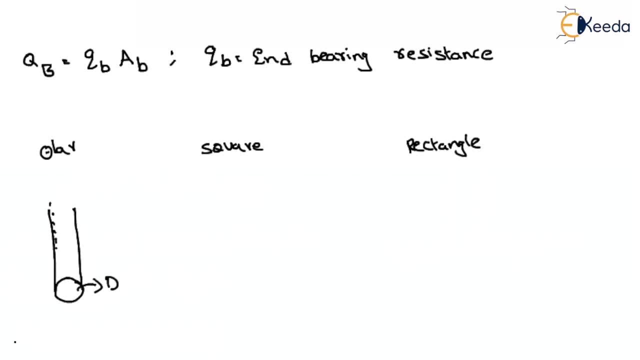 What about the area of the circle with the diameter of the D, then Then n bearing area that can be written as pi by 4 into d square, similarly if it is a square type. so what can we conclude here? let us say each side of the pile is b, whatever the n bearing area that we can be writing as here. 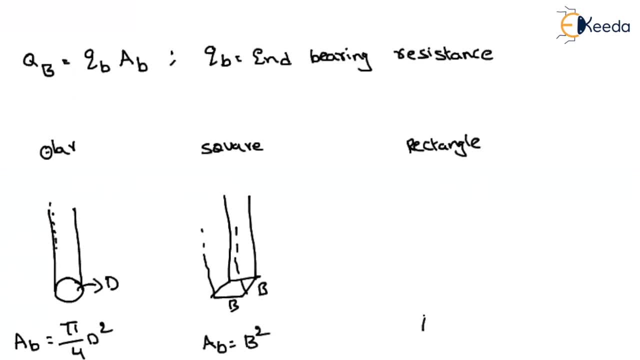 d square. if it is a rectangle, then what can we write here? n bearing area, that will be nothing but a b into d, isn't it? now here i will say: a b has nothing but a n bearing area. the n bearing area is depending upon the column dimensions, isn't it? 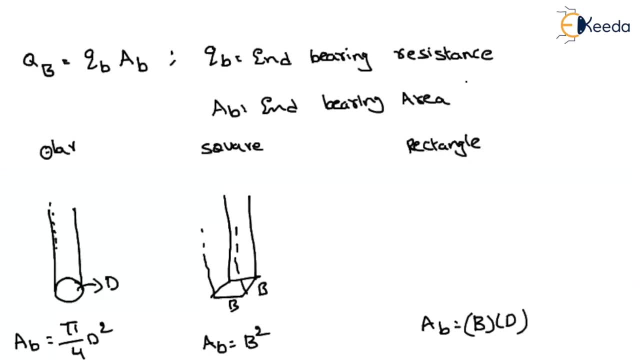 now n bearing resistance is depending upon the type of the soil. so, depending on the pile, you will find out the end bearing area. depending upon the soil, you will find out the end bearing resistance. so this is, what about the evaluation of the end bearing capacity? what about the friction pile capacity? qs is nothing but a. 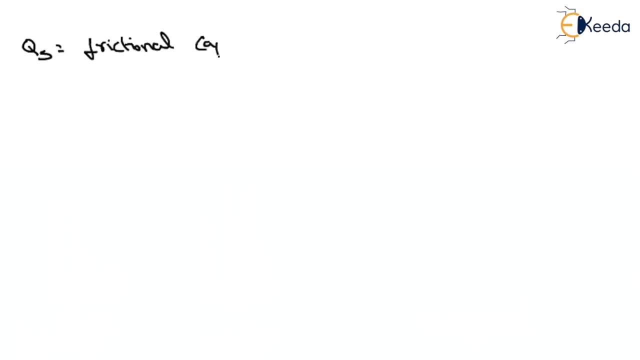 frictional capacity of a pile. similarly, in a similar term, can i express the. this can be represented as a qs into as. whatever the qs can be written as, qs is nothing but a skin resistance between pile and soil. skin resistance between pile and soil. okay, again, this is depending upon the, both pile and also as well as the soil. 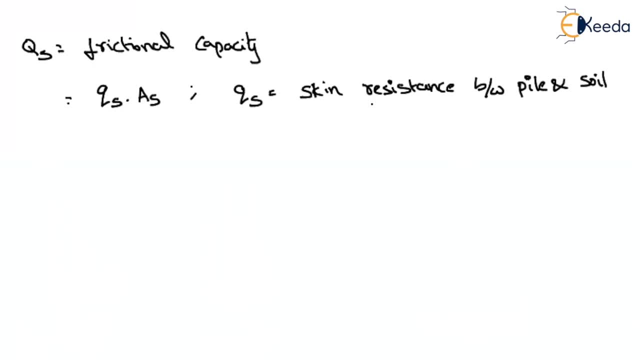 in the previous tjqb. it is only depending upon the type of the soil. if it is a skin friction, it will be dependent upon both soil and the pile. if it is a wood type, it will have one skin friction resistance. if it is a concrete, it will use skill like the 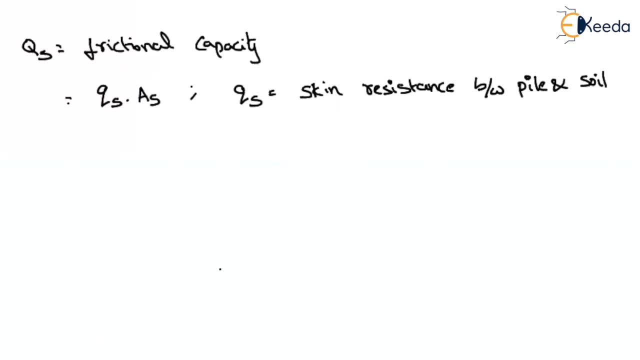 different type of material, you will have the different types of resistance. and what about as area a? is is nothing but a surface area of a pile. surface area of pile. first, let us consider a circular pile. let us consider a circular soil��ing panel soil, soil again. 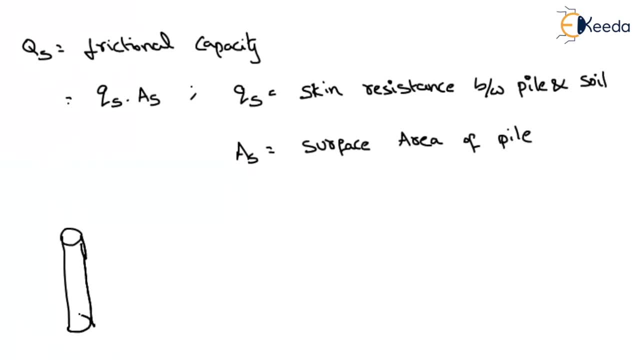 surface area: soil, soil, soil, soil, soil, soil. a circular pile. so what is the surface area? first of all, find out what is the circumference. the circumference is nothing but a pi d into. yeah, that is pi d, right? so what about the length of the pile? that will be equal to, let us say, l. then what about the circumference area? that will be equal. 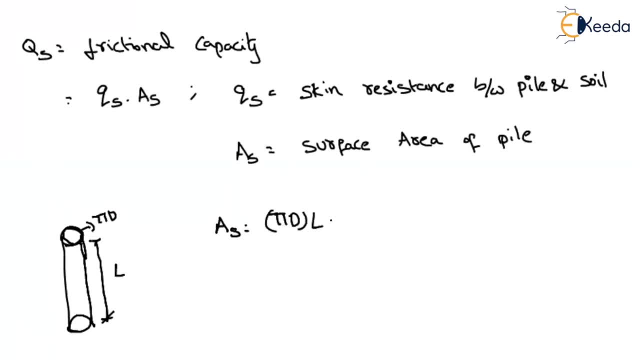 to circumference length, pi d. into what about the total area l? if it is a circular one? what about if it is a square? if it is a square, what about the total surface length? four sides, four sides equal length, that means four into b total length l. so if it is a square, pile, if it is a rectangle, 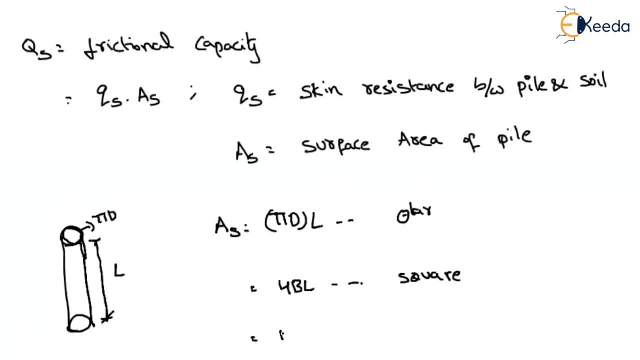 pile, breadth and depth are different. that means we are having two depth, and so two into b, plus d into l. if it is a rectangle, suppose. if i draw the dimensions of the rectangle, it is b. let us say if it is a rectangle, it is b. let us say if it is a rectangle, it is b. let us say if it is a rectangle. 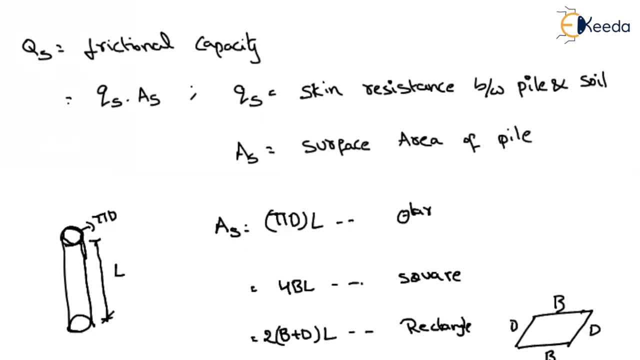 breadth if it is depth. so whatever the circumference length, b plus d plus b plus d, that means two plus two b plus two d if i take common two, two into b plus d over length of l, so whatever the area, l into two, into b plus d, this is for a rectangle. if you are talking about the 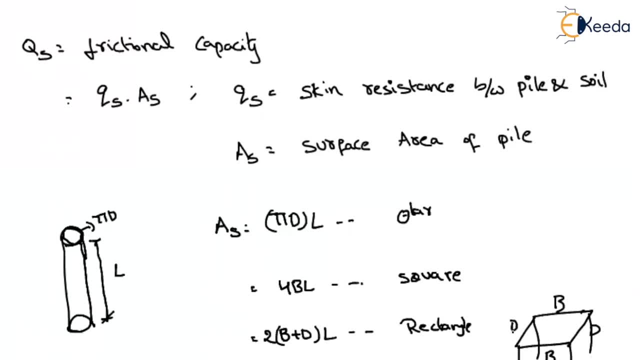 square. all the dimensions are same. so how many sides? we have four sides, that's why four- into b, into l. so, depending upon the type of the file, we have to find out the corresponding surface area and then multiply by the skin friction resistance. then you will get the